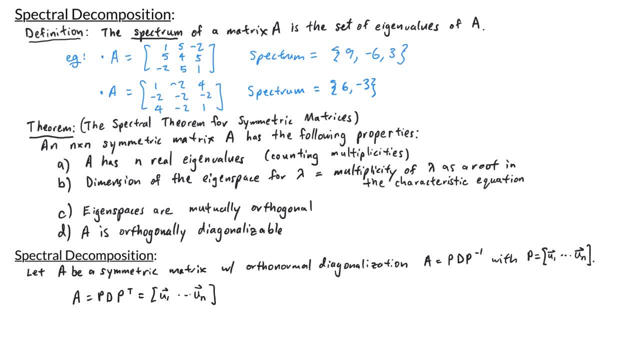 U1 through UN. D is the diagonal matrix with the eigenvalues lambda 1 through lambda n And then P transpose would have rows U1 transpose through UN transpose. Now, multiplying the first two matrices together, we get that this is lambda 1 times U1 through lambda. 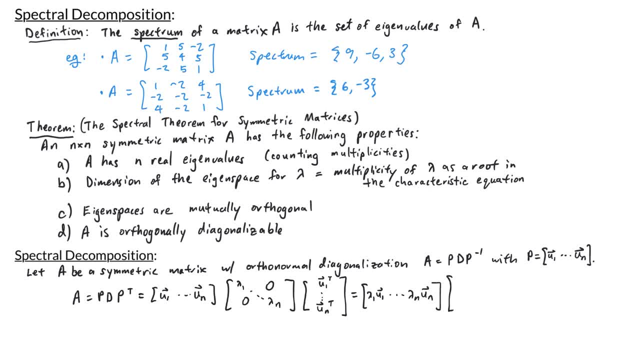 n times UN times P transpose is U1 transpose through UN transpose. Now, using the column row rule for matrix multiplication, we can write this product as lambda one u one times u, one transpose, summed up through lambda n u n times u n transpose. This is what we call the spectral decomposition of A. 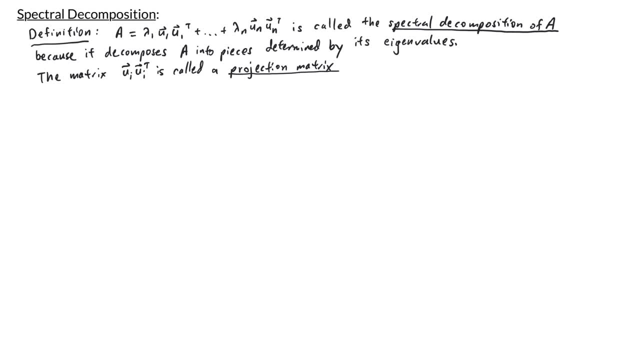 So A written in the form lambda: one times u, one times u. one transpose summed up through lambda n u n u n. transpose is called the spectral decomposition of A, because it decomposes A into pieces determined by its eigenvalues. The matrix u i times u i transpose is called a projection matrix. 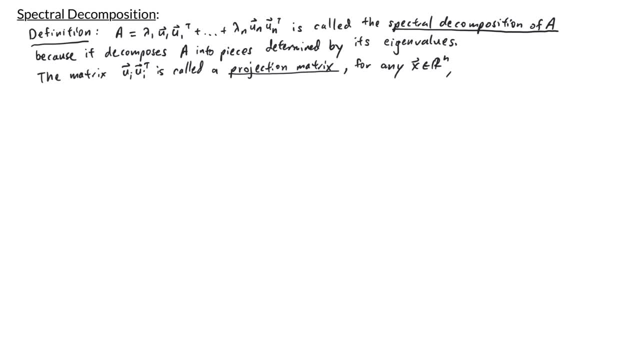 Now, if I take any x in Rn and I multiply it by u i u, I transpose, I get u i u i transpose. times x is equal to u i times u i dot x. Now ui dot x is just a scalar, so I can move it out in front. 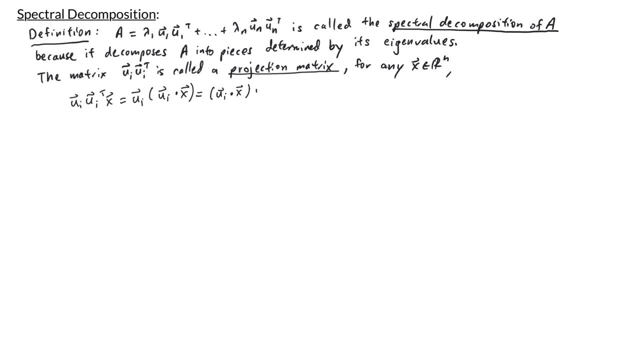 So I have ui dot x times ui, Since ui is a vector with length one, this here is just a projection of x onto ui. So that's why matrices of the form ui, ui transpose, are called projection matrices. Now let's look at some examples of finding the spectral decomposition for. 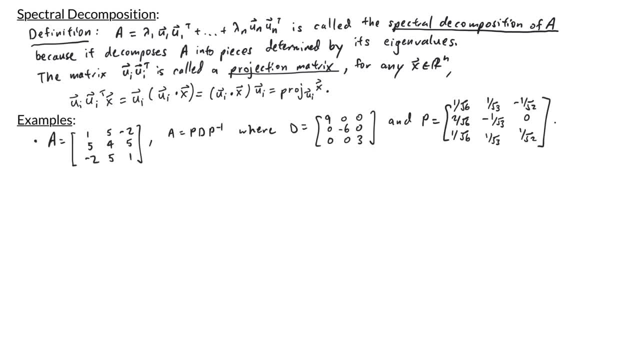 some symmetric matrices. Let's consider this matrix A, with entries 1, 5, negative 2, 5, 4, 5, negative 2, 5, 1.. In a previous video we found that this matrix can be diagonalized. 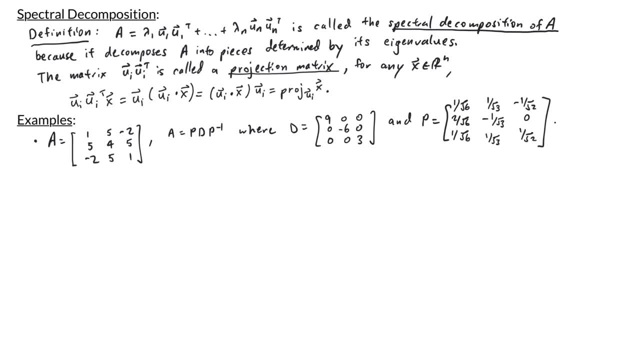 with matrix D equals 9, 0, 0, 0, negative 6, 0, 0, 0, 3, and P is 1 over root 6, 2 over root 6, 1 over root 6, 1 over root 3,. 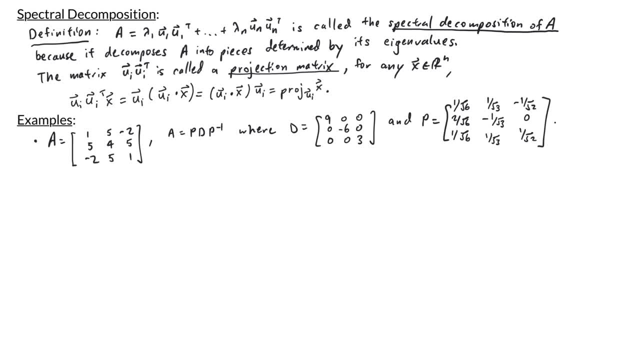 negative 1 over root 3, 1 over root 3, negative 1 over root 2,, 0, 1 over root 2.. In particular, this is an orthonormal diagonalization for A. So if we want the spectral decomposition for A, 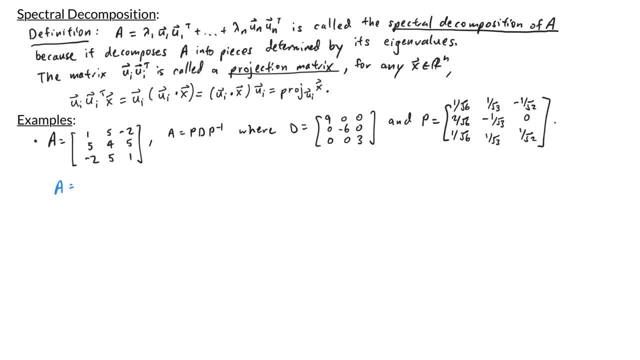 we would write A equals lambda 1, u1, u1 transpose. So our first eigenvalue is 9.. I'll have 9 times the first eigenvector. That's going to be 1 over root 6, 2 over root 6, 1 over root 6, times its transpose. 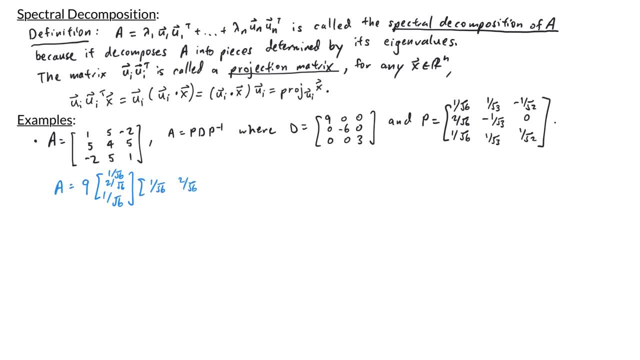 1 over root 6, 2 over root 6, 1 over root 6.. Then add this to the second eigenvalue. that's negative 6, times the second eigenvector: 1 over root 3, negative 1 over root 3, 1 over root 3,. 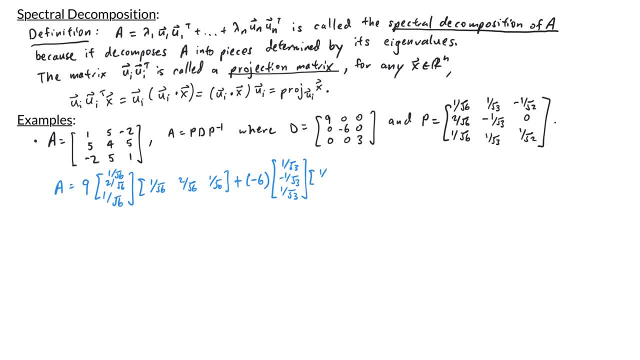 times its transpose: 1 over root 3, negative 1 over root 3,, 1 over root 3, and then, lastly, I have plus 3 times the last eigenvector: negative 1 over root 2, 0, 1 over root 2,. 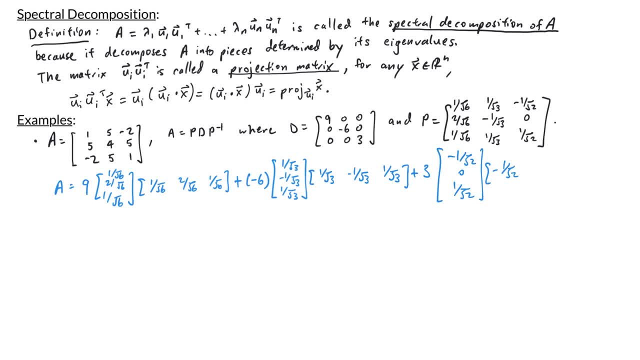 times its transpose negative: 1 over root 2, 0, 1 over root 2.. Multiplying this out, we have 9 times the 3 by 3 matrix, where the top left entry is 1 over root. 6 times 1 over. 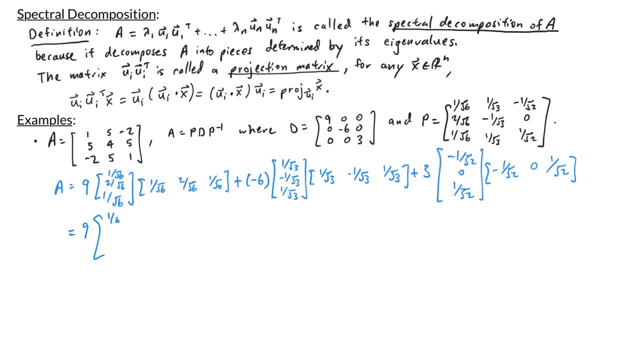 root 6, so that's just 1 sixth. The top middle entry is 1 over root 6 times 2 over root 6, so that's 2 sixths. Then the third entry is 1 over root 6 times 1 over root 6, which is: 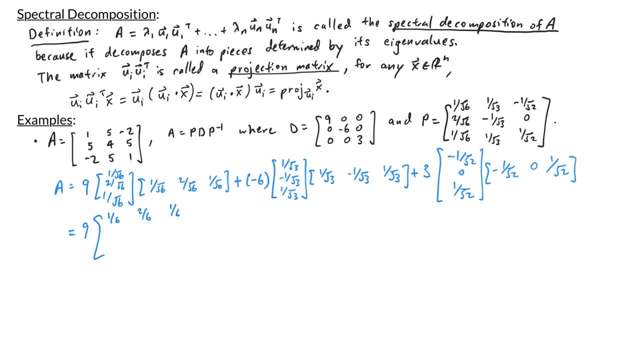 1 sixth. In the middle row we have 2 over root 6 times 1 over root 6, which gives me 2 sixths, Then 2 over root. 6 times 2 over root 6 gives me 4 sixths, Then 2 over root. 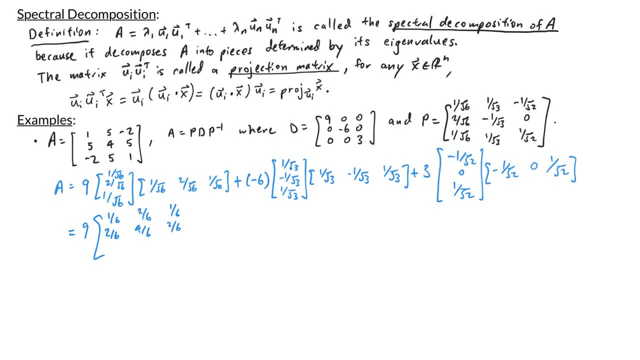 6 times 1 over root 6, I get 2 sixths And in the bottom row I get 1 sixth, 2 sixths and 1 sixth. Then I have minus 6 times the matrix. 1. third negative: 1. 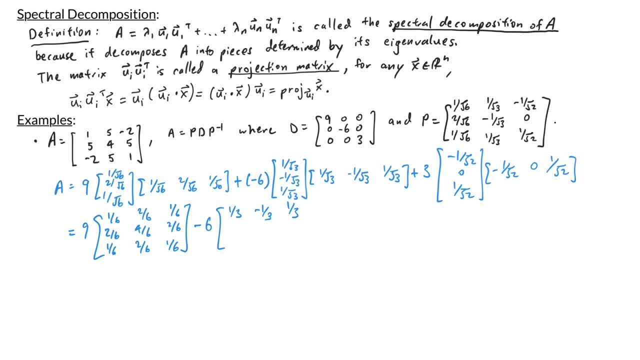 third, 1 third. Then I have negative, 1 third, positive, 1 third, negative, 1 third, and then 1 third, negative, 1 third, positive, 1 third. Lastly, we have plus 3 times the matrix 1. 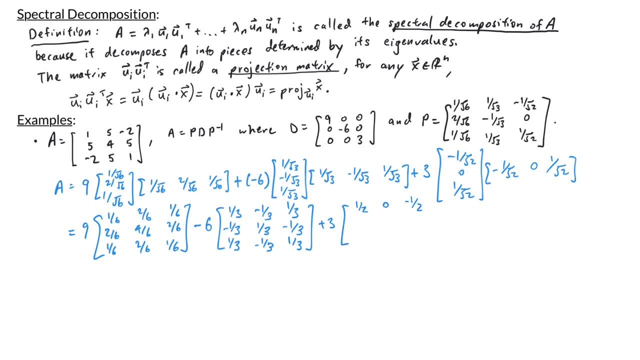 half 0,. negative 1 half, 0, 0, 0, and then negative 1 half, 0, 1 half. So that's the spectral decomposition for A. Let's look at one more example. So here we have the. 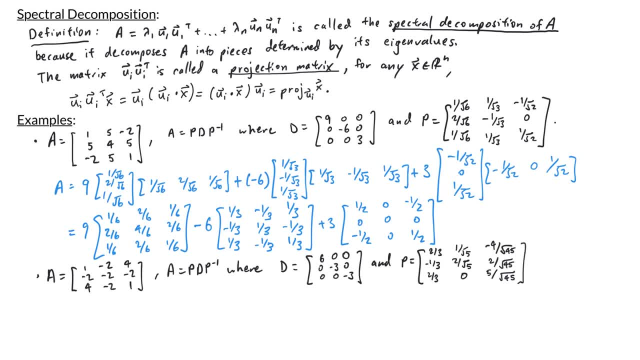 matrix with entries 1, negative, 2, 4, negative 2, negative 2,, 4, negative 2, 1.. Again, we found an orthonormal diagonalization for A in the previous video, with matrix D as 6, 0, 0, 0, negative 3, 0, 0, 0, negative 3, and the matrix P has columns. 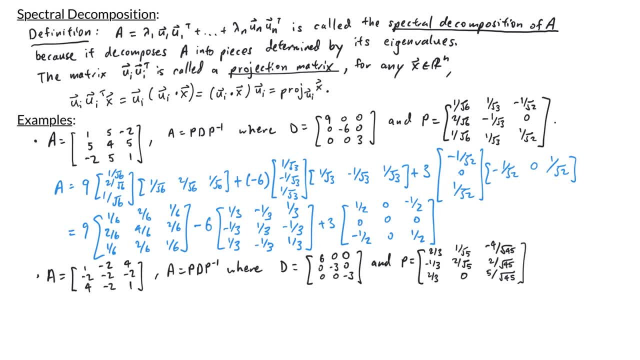 2 thirds. negative 1 thirds: 2 thirds: 1 over root 5,, 2 over root 5, 0, and negative: 4 over root 45,, 2 over root 45,, 5 over root 45.. 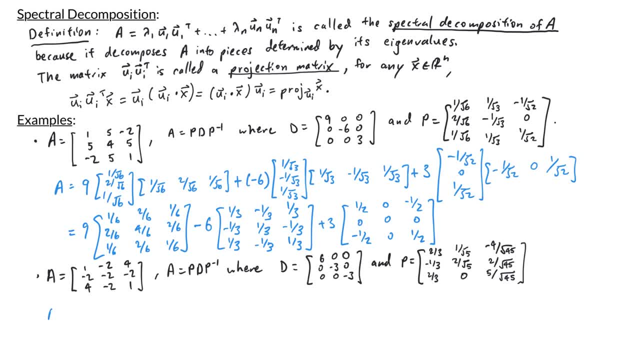 So the spectral decomposition for A would be: A equals the first eigenvalue, which is 6 times the first eigenvector. that's 2 thirds negative, 1 thirds, 2 thirds times its transpose, 2 thirds negative, 1 thirds, 2 thirds. Then we have the second eigenvalue. 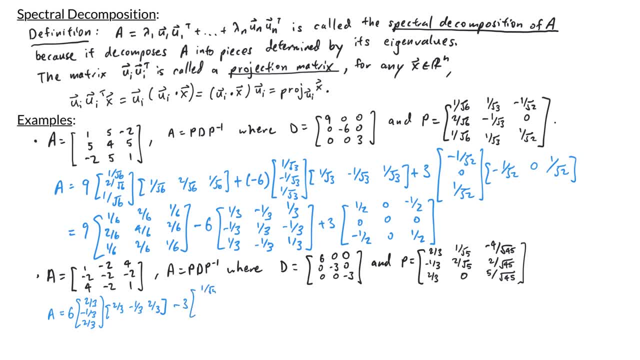 minus 3 times the eigenvector: 1 over root 5,, 2 over root 5, 0, times its transpose: 1 over root 5,, 2 over root 5, 0. Then we have the duplicate eigenvalue negative 3, so we. 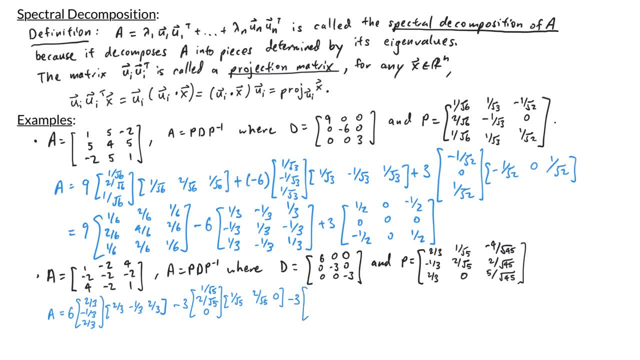 put that here again. So minus 3 times the third eigenvector, negative 4 over root 45,, 2 over root 45, and 5 over root 45, times its transpose: negative 4 over root 45,, 2 over root 45, and. 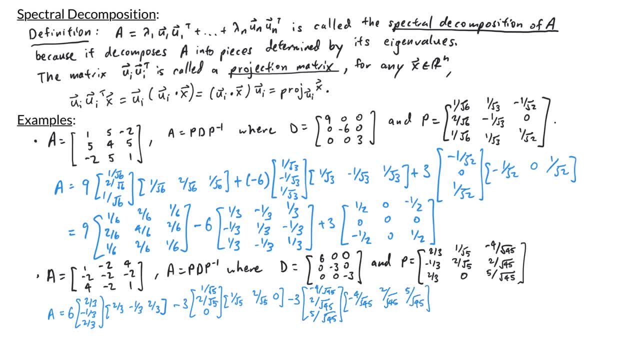 5 over root 45. Multiplying things out, we get that A is 6 times the matrix. 4 ninths negative 2 ninths. 4 ninths negative 2 ninths. 1 ninth negative 2 ninths. 4 ninths negative 2 ninths. and. 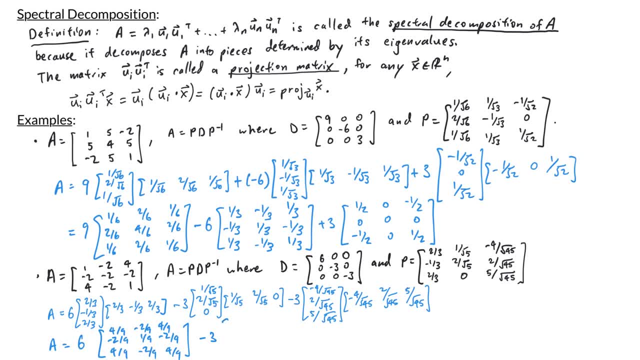 4 ninths minus 3 times the matrix: 1 fifth, 2 fifths: 0,. 2 fifths: 0,. 2 fifths, 1 fifths, 2 fifths, 5 fifths, 4 fifths, 2 fifths: 0,. 2 fifths and 2 fifths and 2 fifths, 1 fifths. 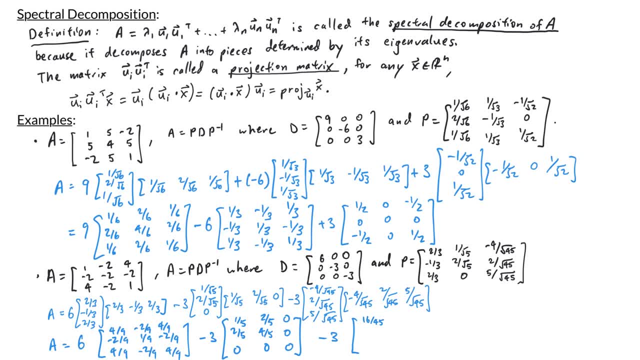 2 fifths and 2 fifths, 2 fifths, 2 fifths, 1 minus 2 ti fourths, negative 3 times the equivalent, which is 4.. And then, lastly, I have, minus 3 times the matrix, 16 over 45, negative 8 over 45, negative 20. 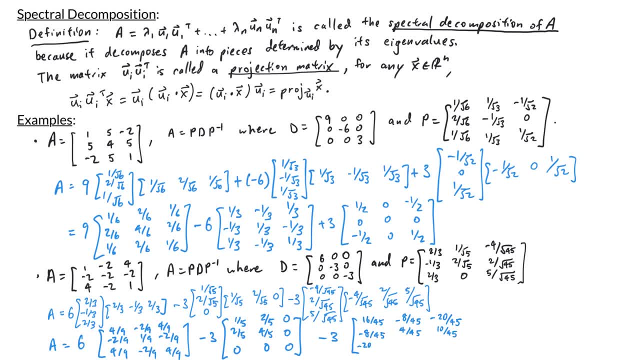 over 45, and then we have negative 8 over 45,, 4 over 45 and 10 over 45, and lastly, negative 20 over 45 and 1 over talent, 1 over Hur crowd, plus 1 over estimate and 1 over